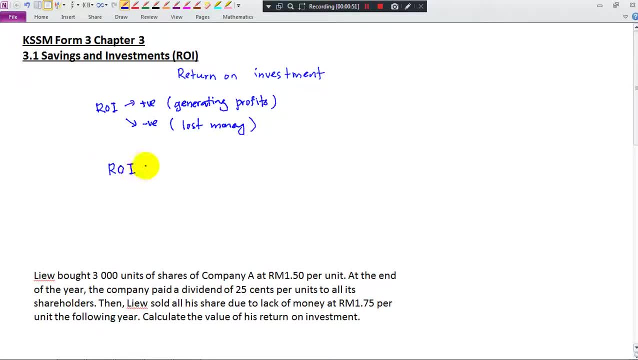 to calculate the ROI return on investment. The formula is the total return. The answer for ROI will be in percentage: How many percent? The total return over the value that you invest? The value of the investment times: 100.. Okay, so the ROI? the answer for ROI will be how: 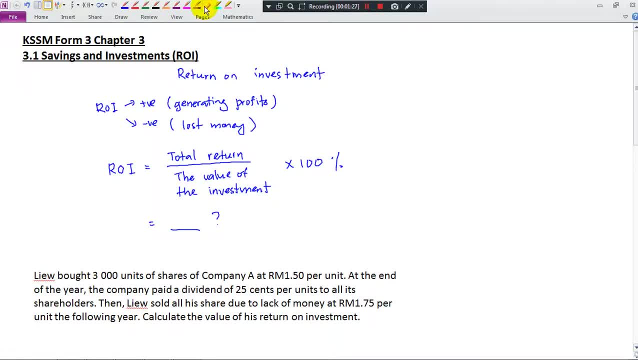 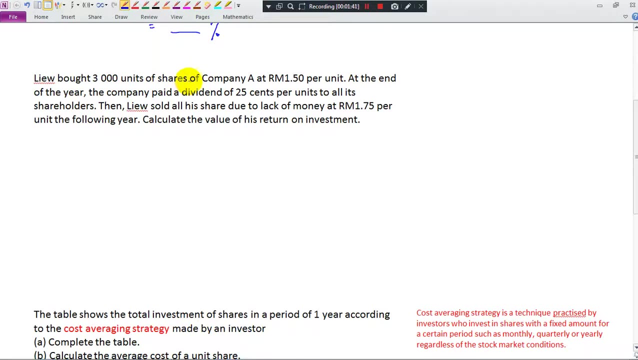 many percent? Okay, Okay, let's look at these questions. Liu bought 3,000 units of share of Company A at RM1.50 per unit At the end of the year. the dividend. the company paid dividends of RM0.25 per unit to all its shareholders. 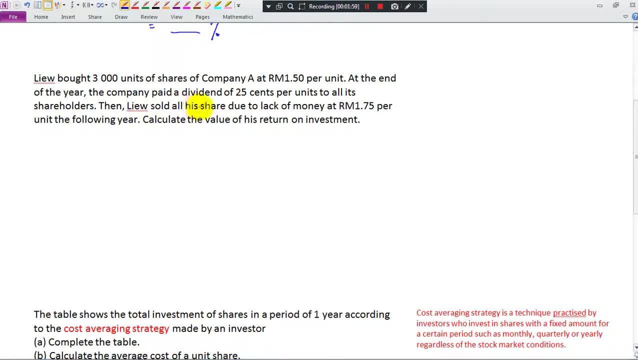 then you shows all his share, due to lack of money, at $1.75 per unit of the in the following years they calculate the value of his return on investments. means that we need to calculate the ROI. okay, first we calculate the amount of money he invests, the initial capital, the course 3,000 units. 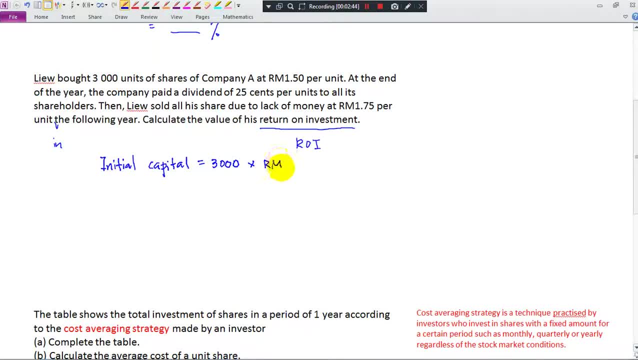 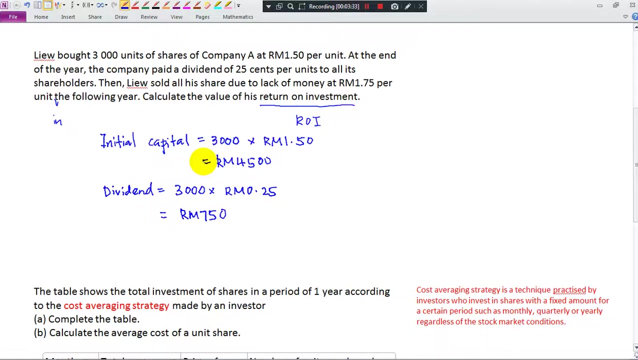 one unit, one ringgit and 50 cent. okay, just press the calculator. this will give you four thousand and five hundred. okay, now we cut in the dividend, receive one unit, 25 cent. right, so now we have. he has three thousand units times 25 cent, seven, five, oh, okay. so after that he sold all his share in at a price of one. 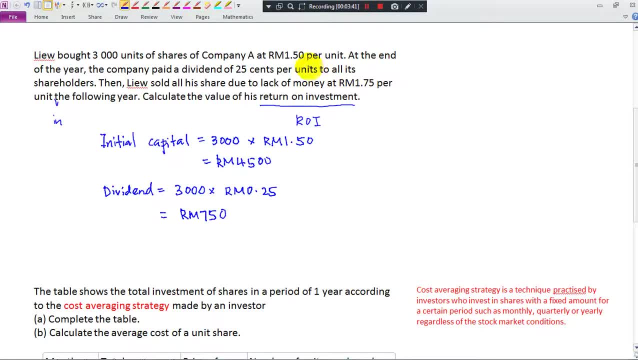 ringgit and 25 cent. actually, he is getting money right when he bought this one ringgit and 50 cent per unit. when he sell, he sell, he sell in at a price of one ringgit and 75 cent. okay, so happy the game, oops. 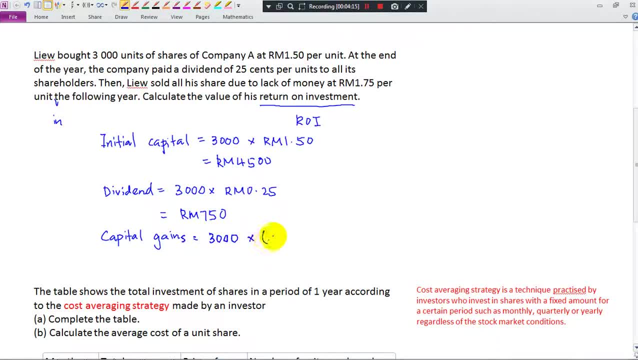 3000 units. okay, so this is. the selling price is one ringgit and 75 cents minus two. the initial price 1 ringgit and 50 cent. so means that one unit he earns 25 cent, 7, 5, 4. Okay, so the ROI still remember the formula. 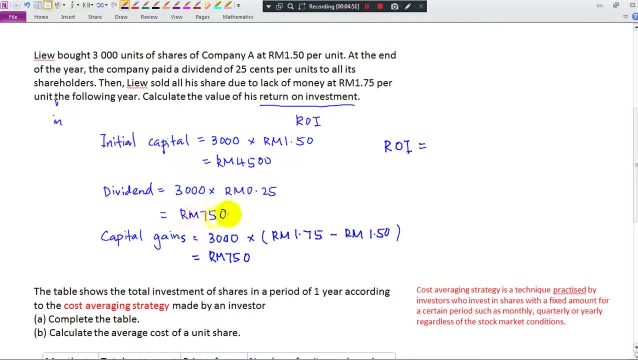 It's a total return from the dividends Receive: seven hundred and fifty ringgit. when he sells The share, he earned another seven hundred and fifty ringgit. The money invested by him is Four thousand and five hundred. so how many percent He earned? what is his ROI, which is press the calculator? 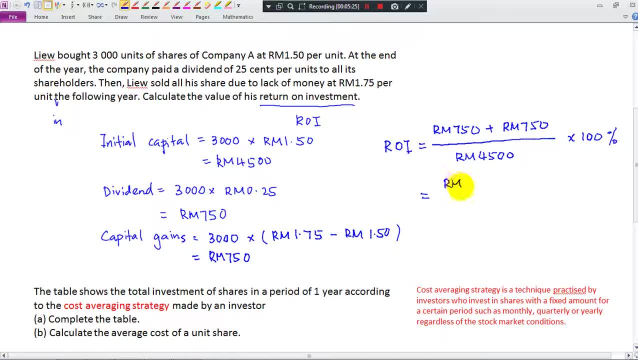 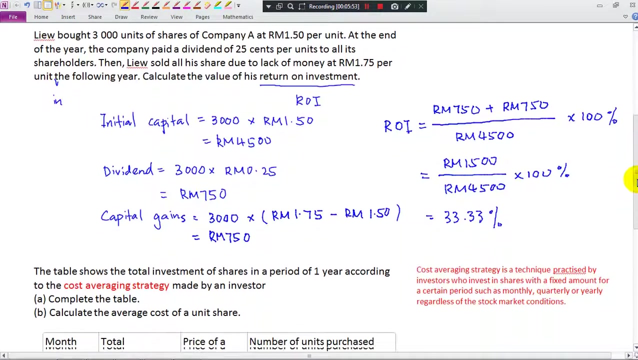 So. So total earning is one thousand five hundred out of four thousand and five hundred. So still remember, just I told you the ROI is in percentage. so divided by four or four, five or 100, Thirty three point three, three percent. Okay, let's look at this one. 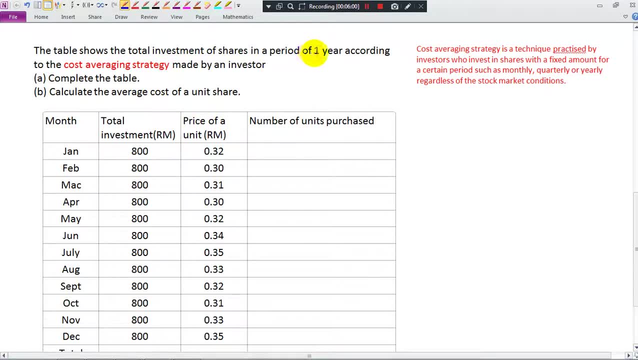 The table shows total investment of share in the period of one years according to the cost averaging strategy. Okay, this one the definitions over here. cost averaging strategies is a technique practice practiced by Investor who invest in a share with a fixed amount for a certain period. They see every month spend eight hundred ringgit. 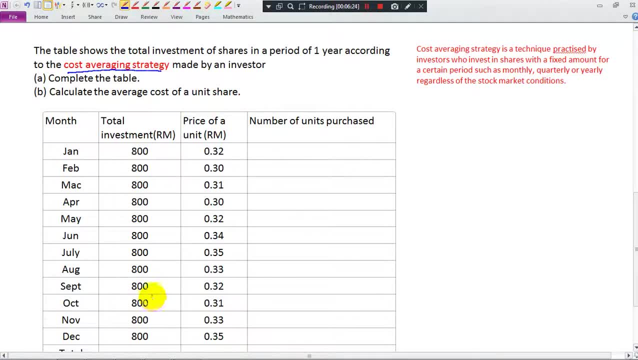 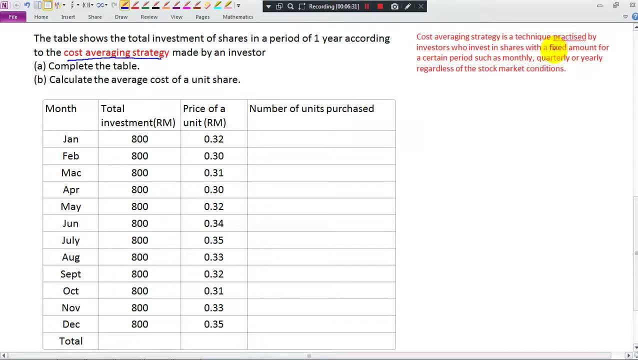 Instead of spend one lump sum to buy all share, Okay, Okay, let me complete this one first with a fixed amount. fixed amount For a certain periods, such as monthly, quarterly or yearly, regardless of the stock market condition. Okay, Now, how do we solve this question? 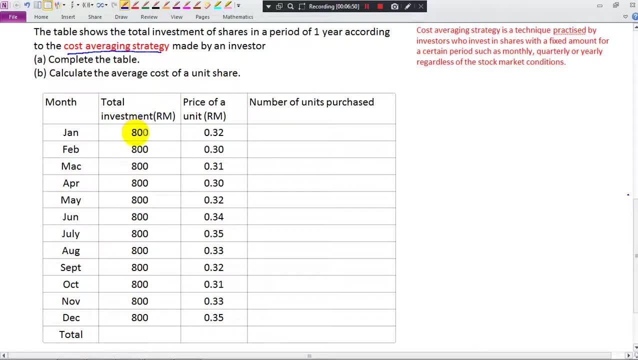 Every month. the investor spent eight hundred ringgit to buy the share and you will notice that a share price of the unit keep on changing. First we need to complete the table number of unit purchase. So how to calculate the number of unit purchase is actually very easy. So this is. 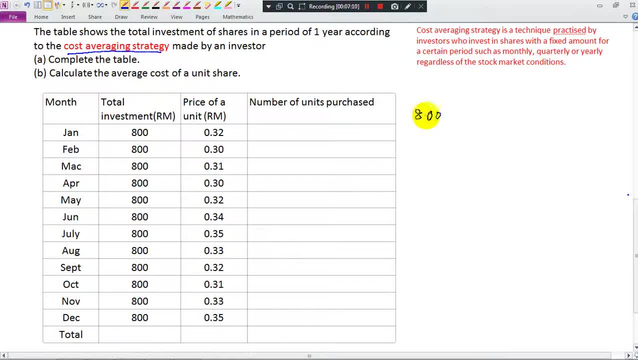 800, right or sorry? Yeah, yes, correct. 800 ringgit. One unit is 0.32. They press the calculator: eight hundred divided by zero, point three to which will give you 2500 units. how about this one? they do the same thing. 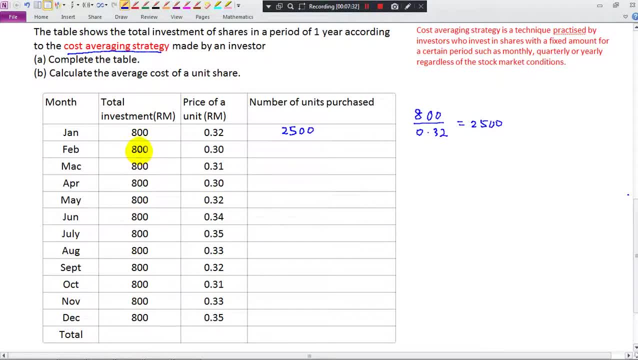 for the rest, take this one total investment divided by the price of a unit share. okay, these are the number of units purchased by him. okay, so we need complete the table, the total here, the money, the total money that invested by him, because you are eight hundred times 12, 12 month, which is nine thousand nine. 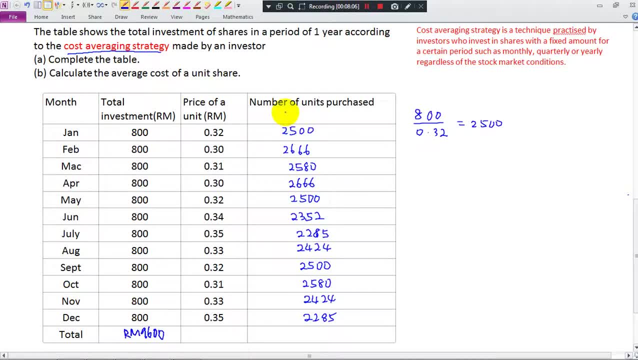 six, four, four. okay, the total number of units purchased by him is, plus all this number together, two, nine, seven, eight, two. okay, let me check again, correct, not okay, correct: calculate the average cost of a unit share. so how do we calculate average cost of a unit share? so the total amount spent here is nine thousand and six hundred, right, nine.